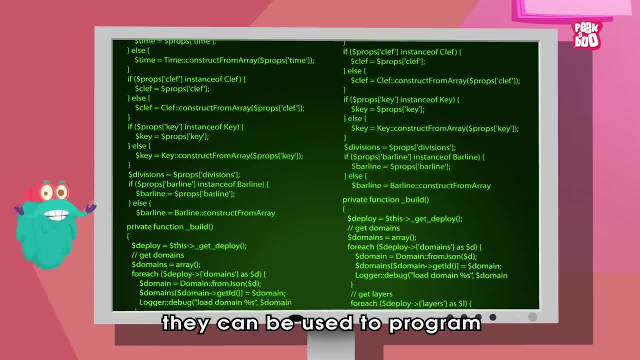 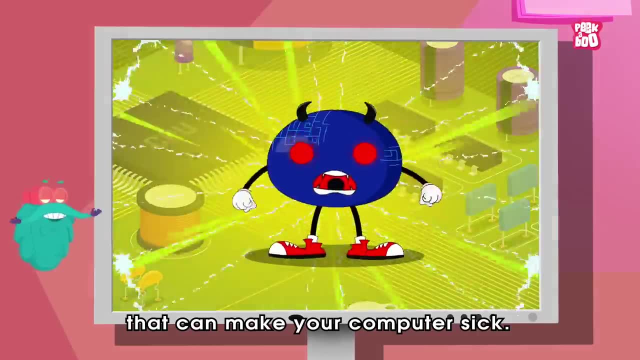 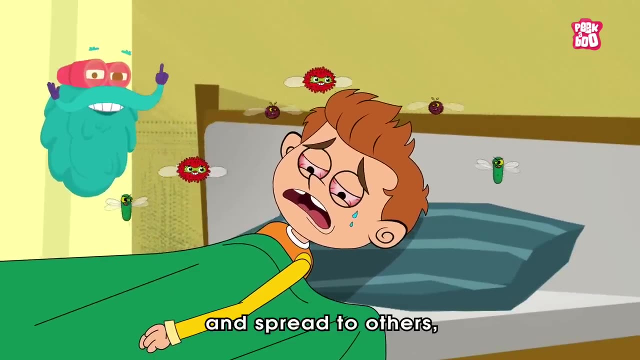 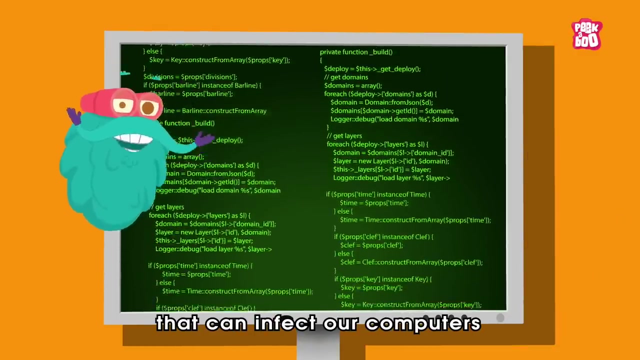 helpful. however, at times they can be used to program harmful software, called viruses, that can make your computer sick. Yes, just like how a living virus can make us sick and spread to others, computer viruses are like small, Invisible creatures that can infect our computers and other similar devices. 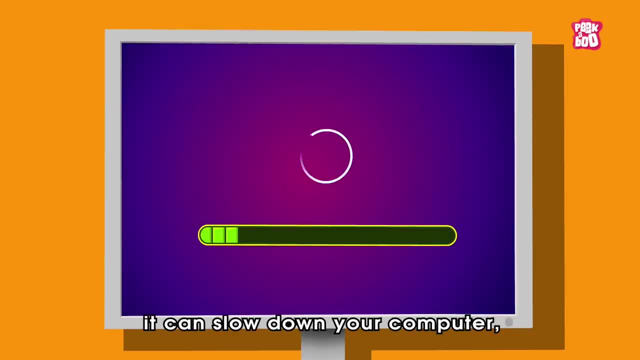 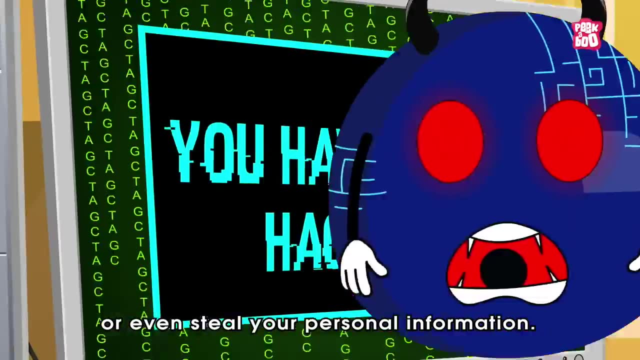 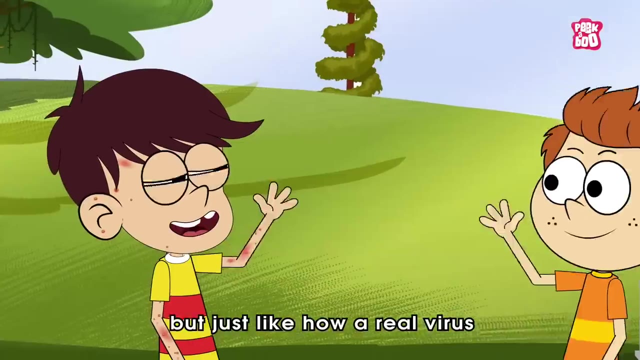 Once a virus is inside your device, it can slow down your computer, make it freeze or crash, delete your files or even steal your personal information. Not only that, but just like how a real virus can spread from one person to another, the computer virus can also spread to others. 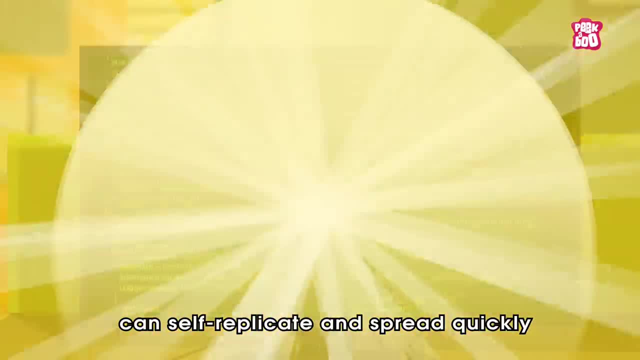 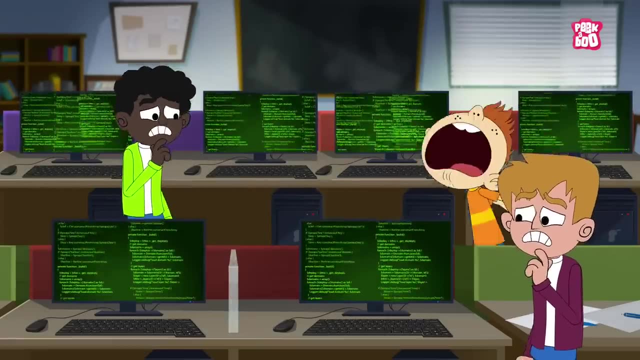 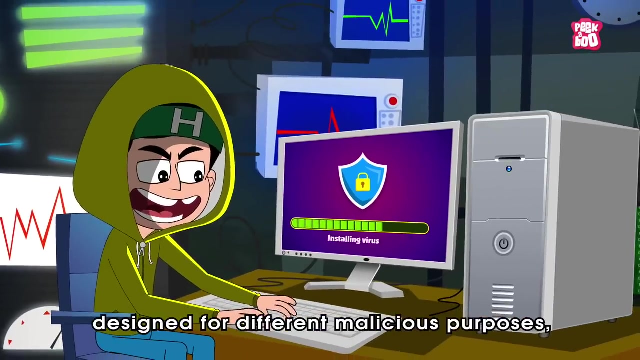 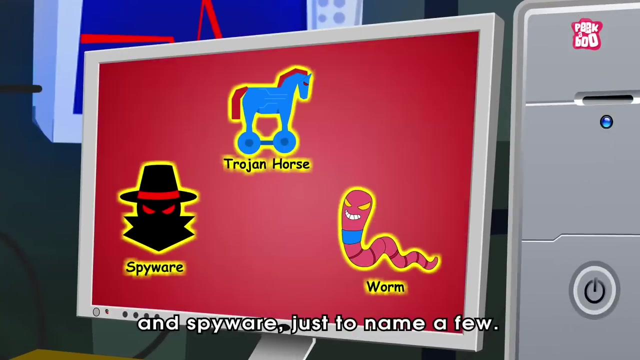 A virus can self-replicate and spread quickly from one computer to another, causing havoc on a large scale. And, believe it or not, there are possibly thousands of viruses designed for different malicious purposes, like Trojan horses, worms and spyware, just to name a. 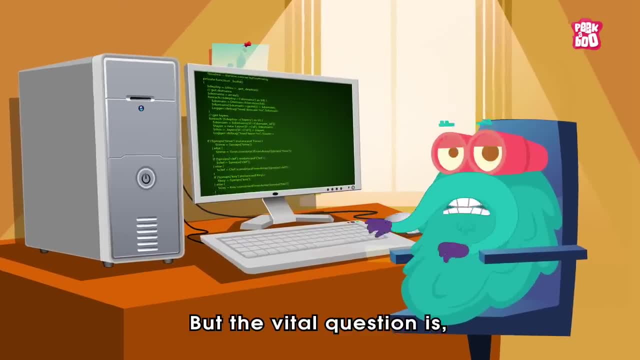 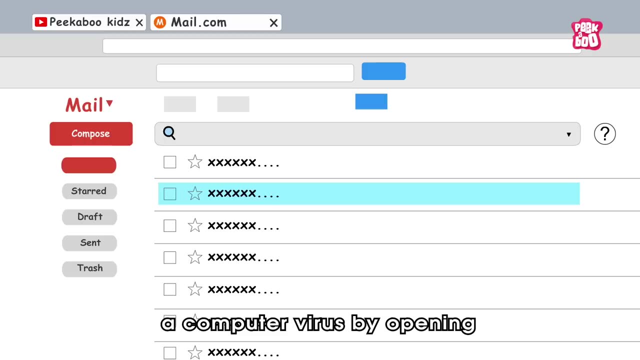 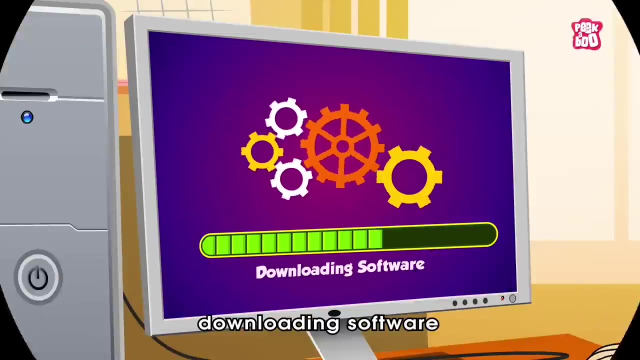 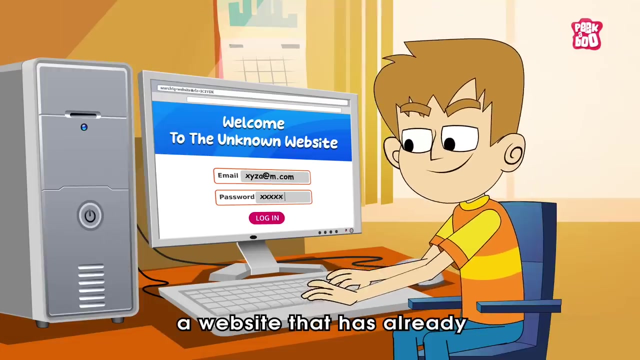 few. But the vital question is: how can our devices? devices get infected? Well, you can accidentally catch a computer virus by opening an email attachment from someone you don't know, downloading software from an unsafe platform, or by visiting a website that has already been infected with a virus. 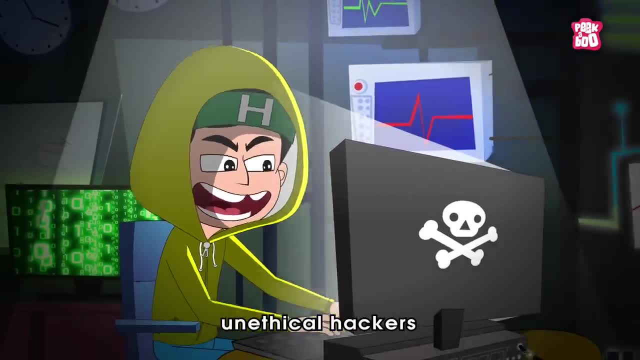 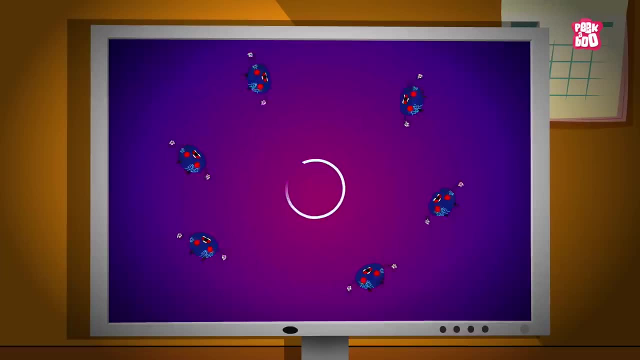 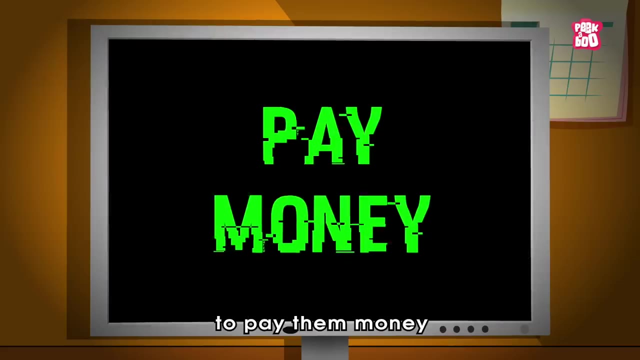 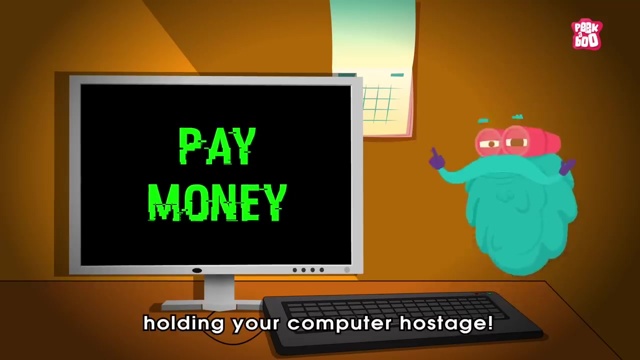 Not only that, but sometimes unethical hackers can sneak into your computer and deliberately put a virus on it. This virus can make your computer stop working and the hackers might ask you to pay them money to fix it. It's like a bad guy holding your computer hostage. 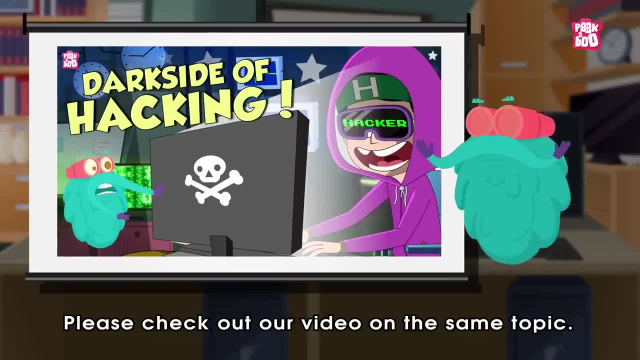 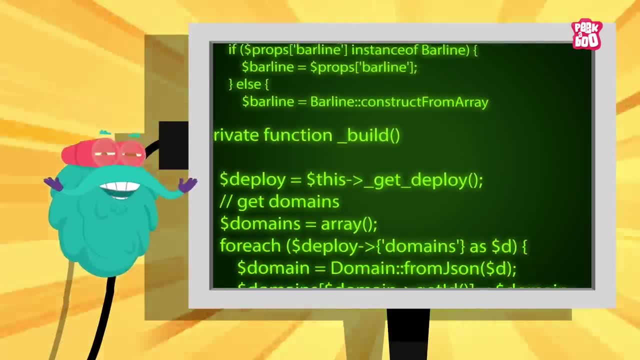 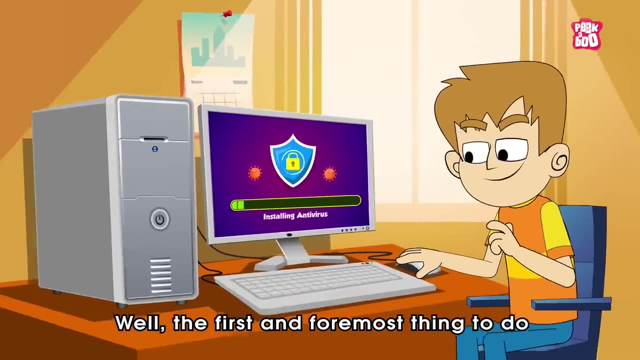 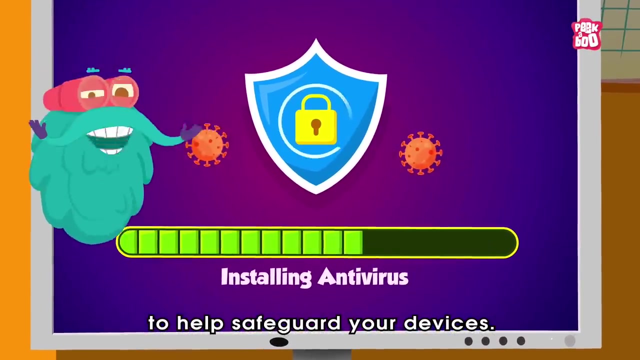 To stay safe from hackers. please check out our video on the screen. Now here comes the most important question: What can we do to protect ourselves from these corrupted codes? Well, the first and foremost thing to do is install antivirus software to help safeguard your devices.